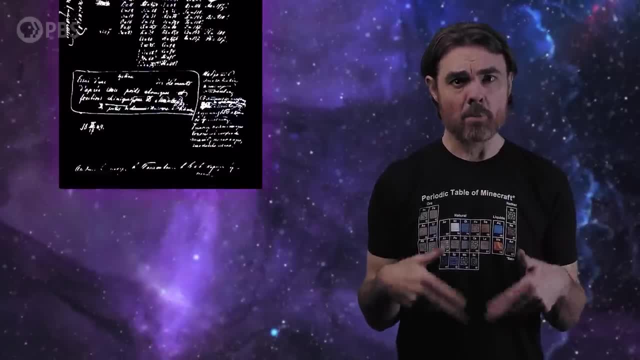 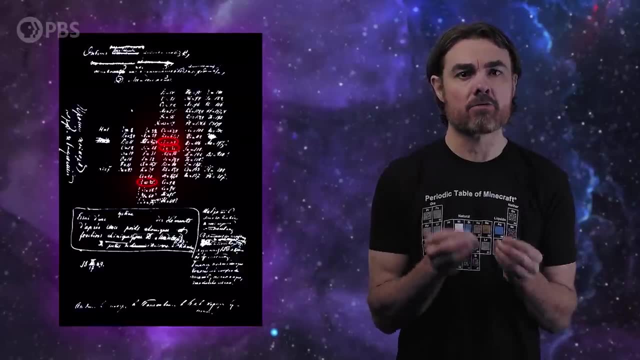 filling the next shell up. Although he didn't know about protons, Mendeleev did notice gaps in his periodic table. He correctly interpreted these as four elements that had yet to be discovered. He was even able to predict many of their properties. 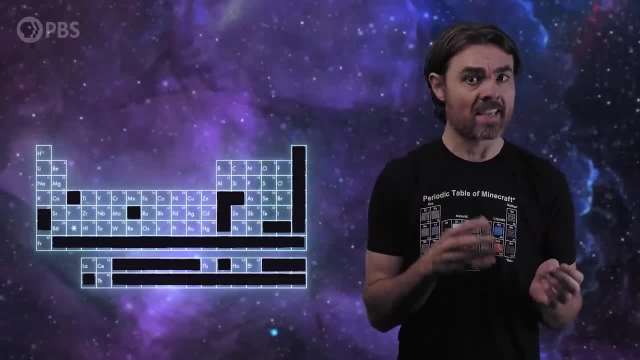 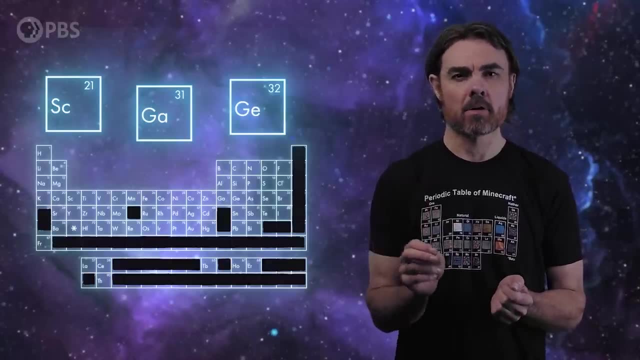 Over time, three of these elements were discovered and the gaps were filled with scandium, gallium and germanium, But there remained a missing element Right between molybdenum and ruthenium, which we figured out had to correspond to a nucleus. 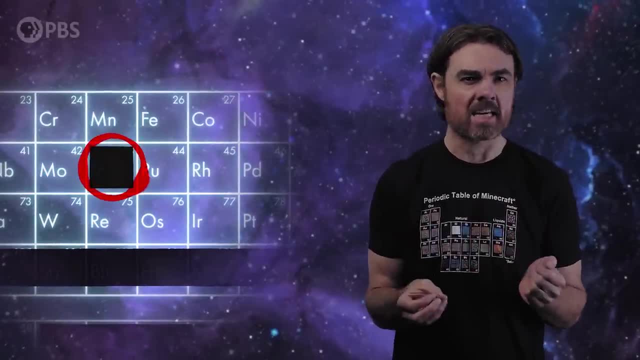 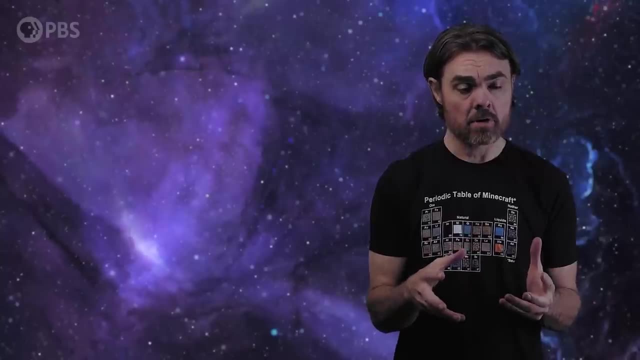 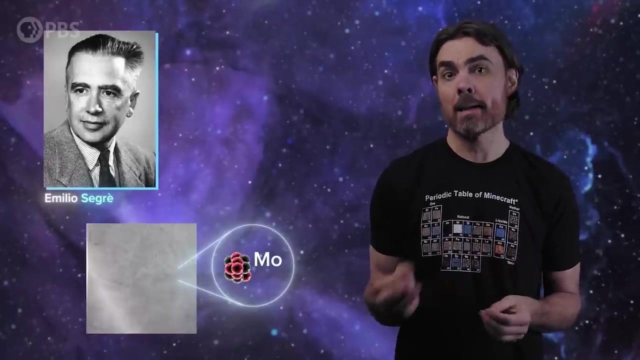 with 43 protons. For seven decades, chemists searched for element 43, but it was nowhere to be found in nature. It was eventually discovered, but not in nature. In 1937, Italian physicist Emilio Segre got hold of some molybdenum foil that had been 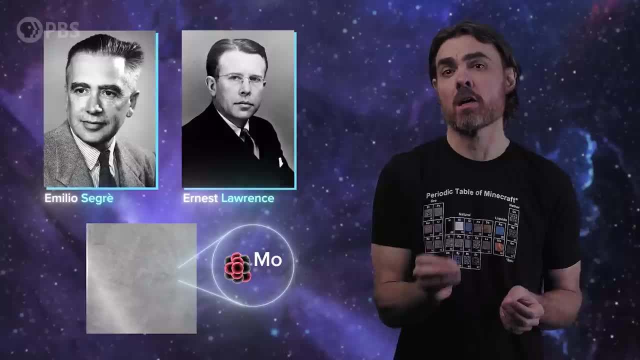 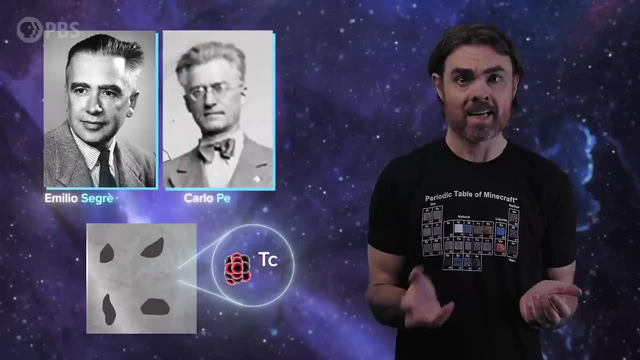 part of Ernest Lawrence's newly invented cyclotron particle accelerator. The foil had been rendered radioactive in the accelerator, and Segre and his colleague Carlo Perrier were able to show that some of the molybdenum had gained a proton transmuting. 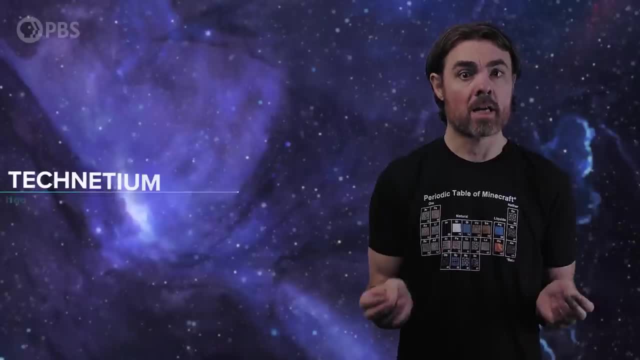 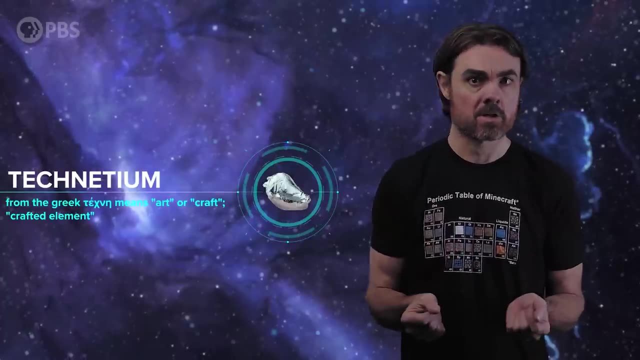 it into element 43.. They named the new element technetium after the Greek word for art or craft, so in a sense its name means crafted element. It's a silvery-grey metal with chemical properties somewhere between manganese and rhenium, the 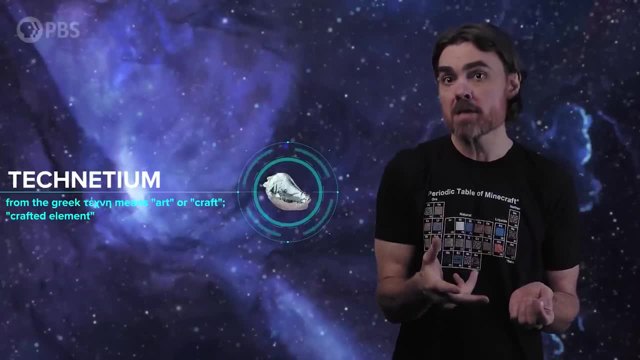 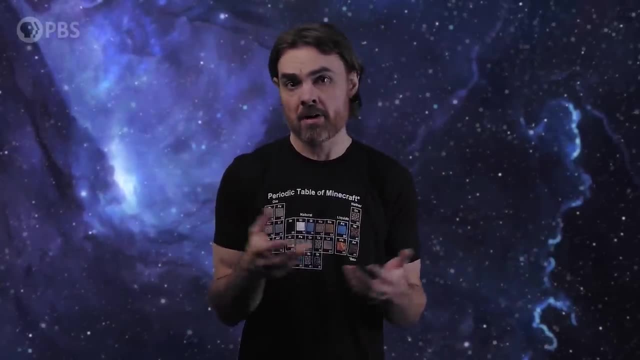 elements above it And you can see how it's been used in the periodical table. So why did we have to produce technetium artificially when all the other elements can be found in nature? Well, actually, technetium is produced in nature, just like other heavy elements in. the core of massive stars. Those elements eventually find their way into planets which form from the guts of those stars after they explode as supernovae. But technetium is so unstable that by the time the earth has become a planet, it's gone. 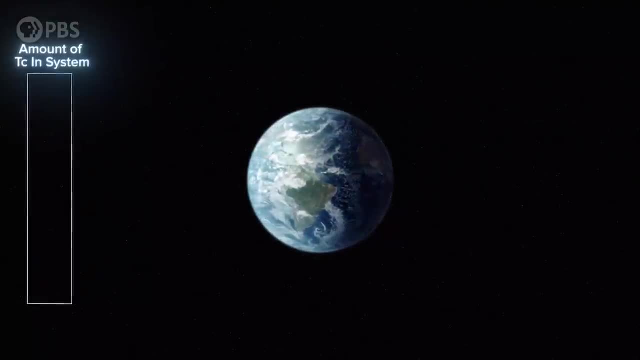 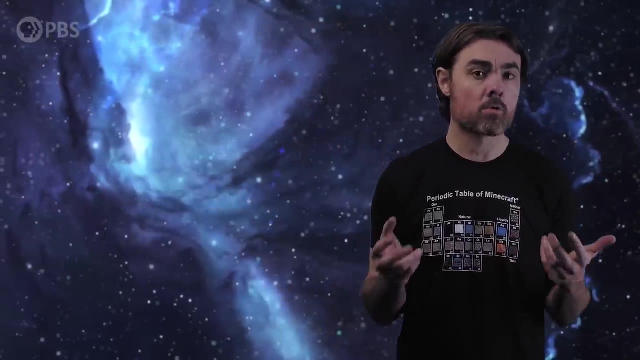 The earth pulled itself together from the detritus of dead stars. all the technetium was long gone. You're probably familiar with the idea that elements can be unstable. A more common term is radioactive, which we tend to associate with very heavy elements. 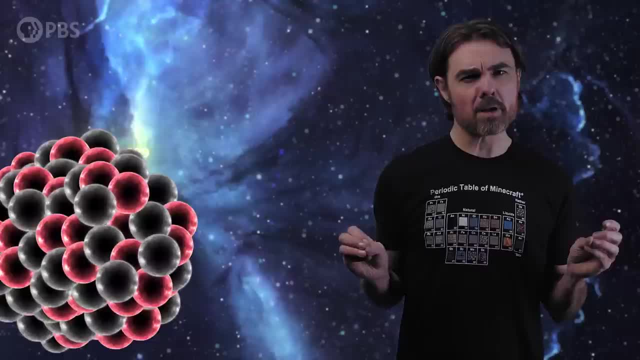 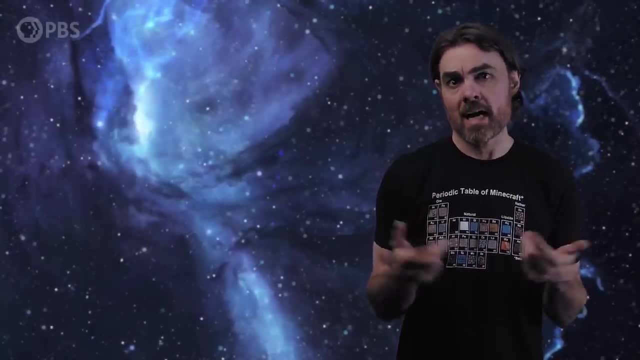 like uranium and plutonium. For those the instability sort of makes sense. Their nuclei are enormous, so you might expect they'd have trouble holding themselves together. But actually any element on the periodic table can be unstable, Or more precisely, they're not. 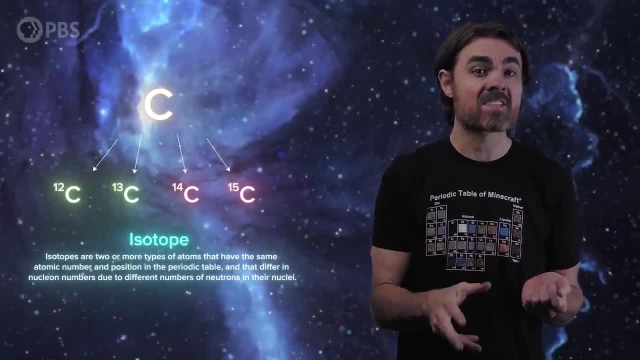 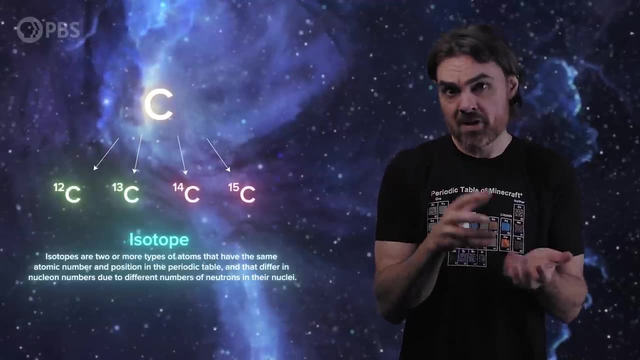 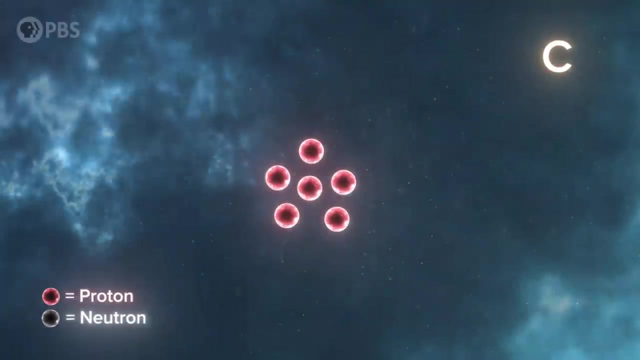 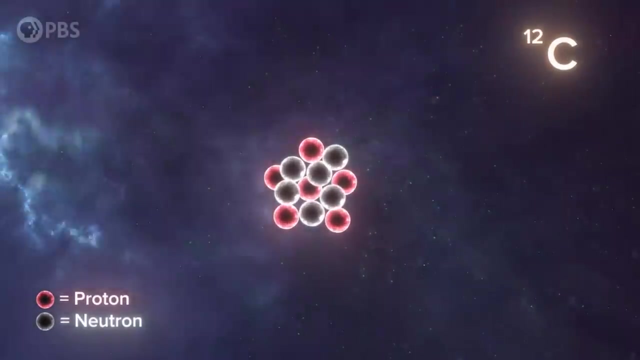 More accurately. every element on the periodic table has unstable isotopes. Isotope is the word for different versions of the same element, but with different numbers of neutrons. For example, a carbon atom has 6 protons in the nucleus. The isotope of carbon that also has 6 neutrons is called carbon-12 for its 12 total nucleons. 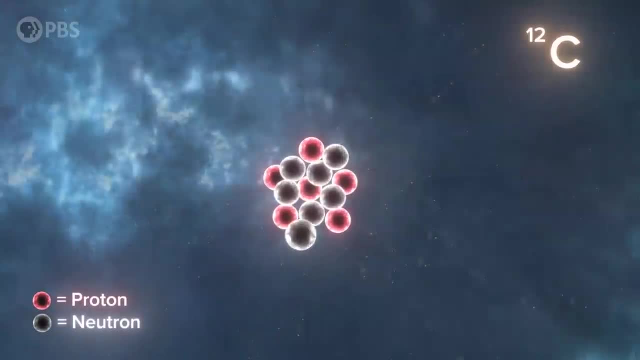 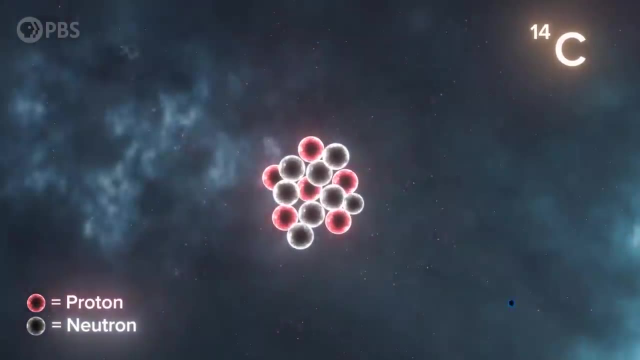 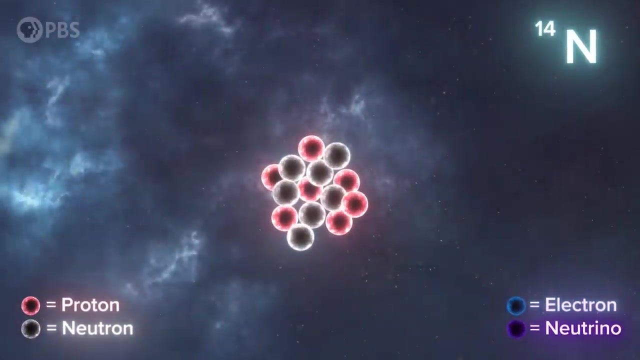 and it's perfectly stable. An atom with 6 protons and 8 neutrons is stable. It has a tendency for one of its excess neutrons to transform into a proton after ejecting an electron and a neutrino, which transmutes it into nitrogen. 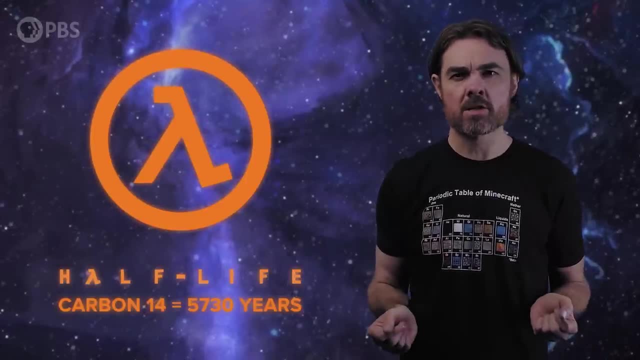 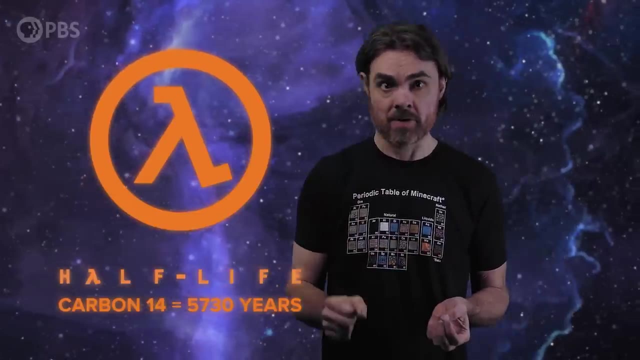 The half-life of carbon-14 is around 5,700 years, although we do encounter it in nature because it's created when cosmic rays hit nitrogen nuclei in the atmosphere. We say carbon-14 is an unstable isotope of carbon. We say carbon-14 is an unstable isotope of carbon. 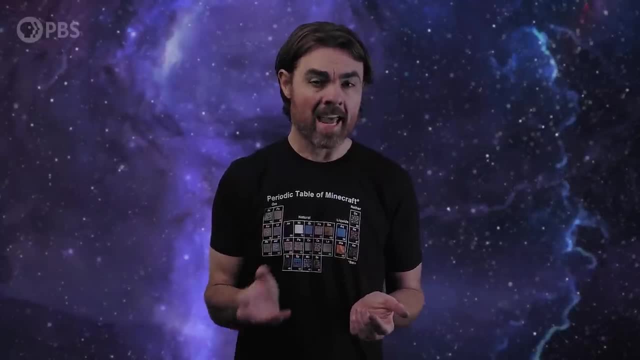 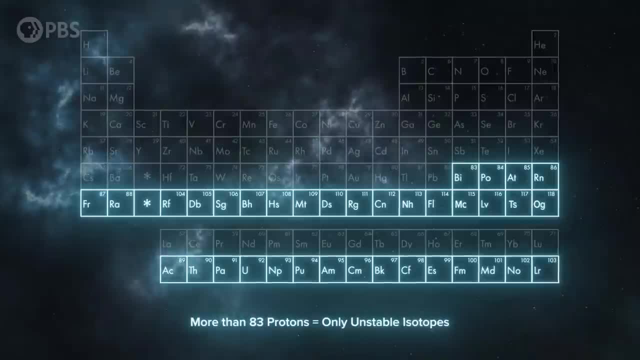 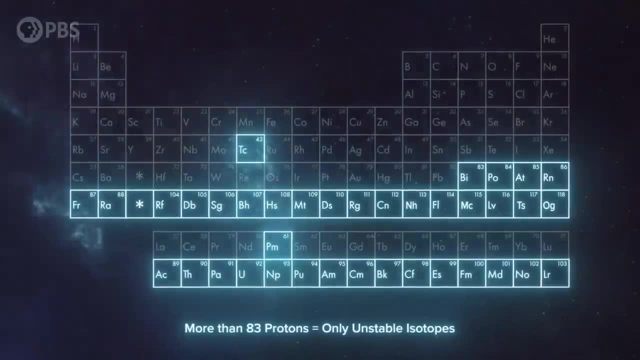 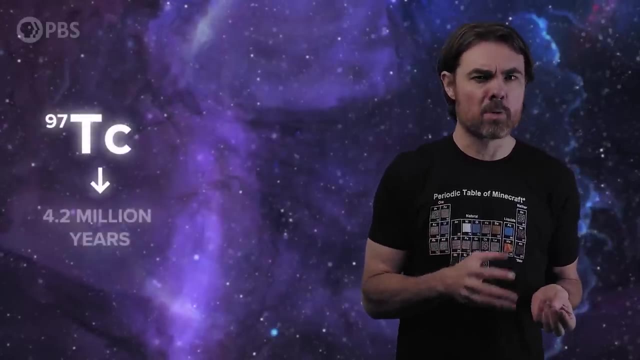 For example, any with more than 83 protons, But also weird exceptions like technetium, as well as element 61, promethium, And there are shades of instability. For example, technetium-97 has a half-life of 4.2 million years, while technetium-96. 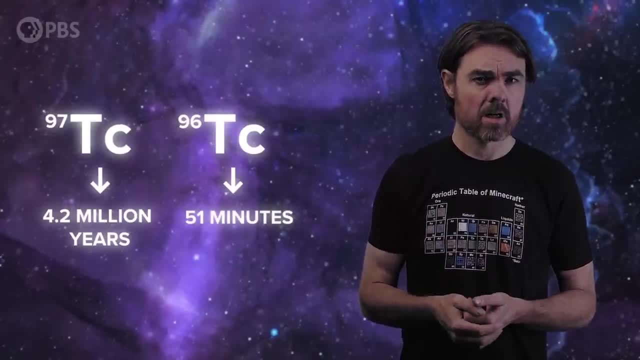 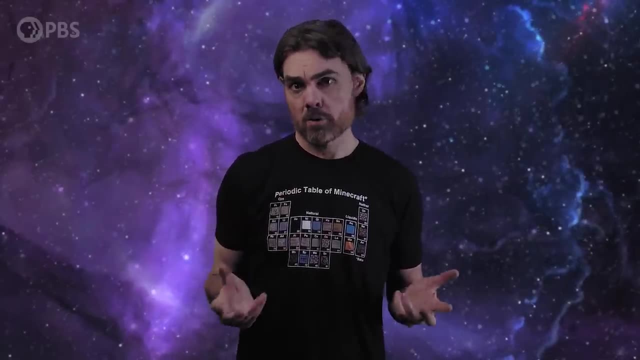 has a half-life of 51 minutes. minutes Larger atomic nuclei tend to yield fewer stable isotopes and have shorter half-lives. Elements with more than 118 protons decay so quickly that we've never been able to detect one in the lab. 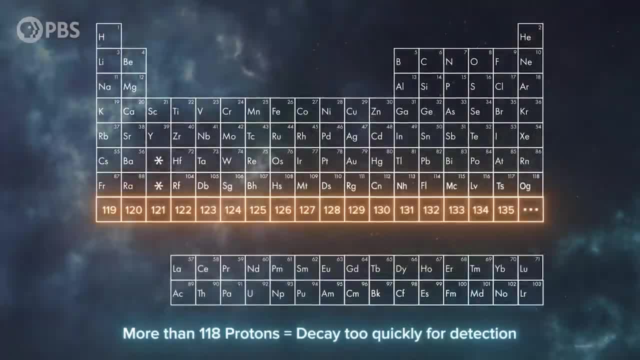 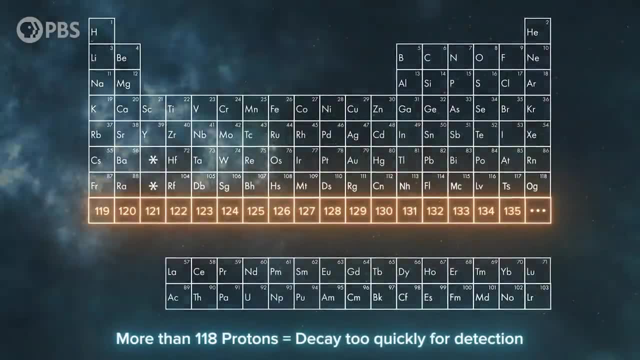 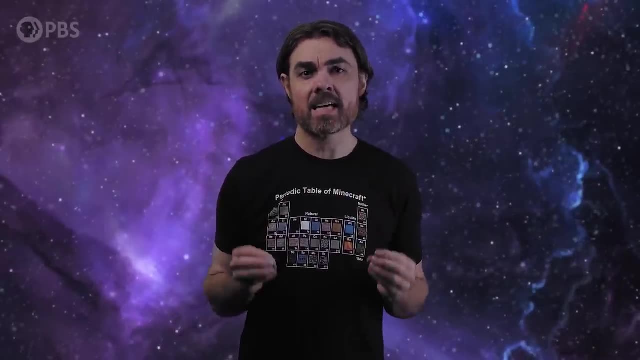 Ultimately, stability depends on the balance between protons and neutrons in the nucleus. You might think that after a century and a half of thinking about nuclear physics we'd have all this figured out, But actually the dynamics of the atomic nucleus are so complicated that it takes sophisticated 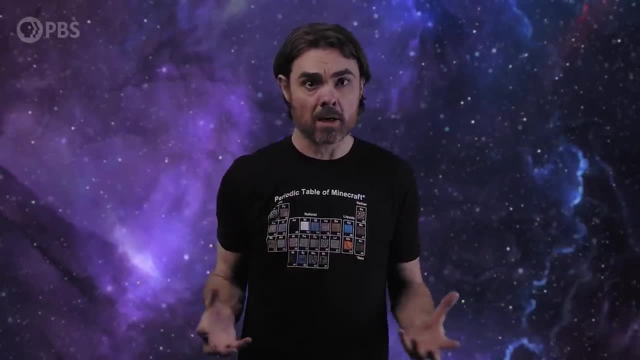 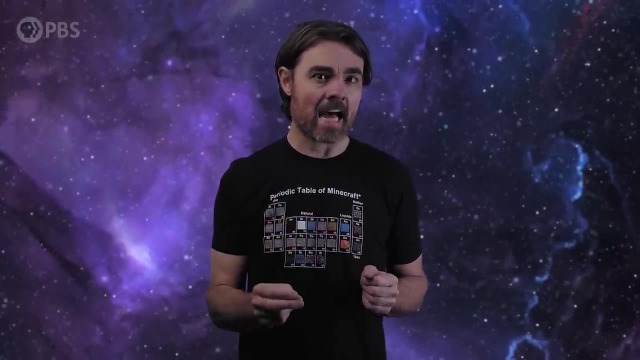 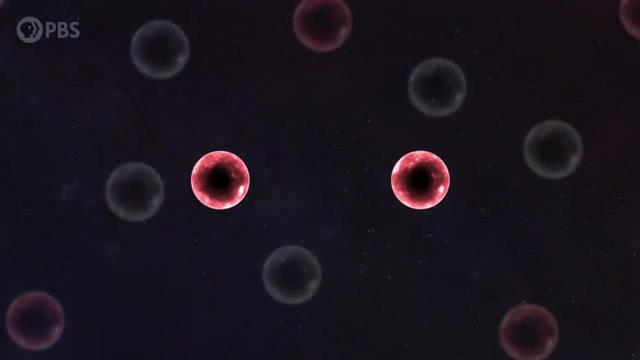 computer modeling to understand any but the lightest elements, And many mysteries still remain. But we're getting there. So let's see if we can at least lay out the competing influences at work. An atomic nucleus is a place of extreme forces in delicate balance. 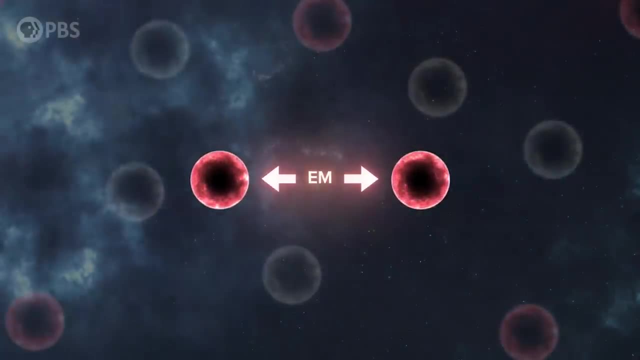 On the one hand we have the electromagnetic force. It's trying to force apart all those positively charged protons and the strength of that force is great due to the proximity of the protons. On the other hand, we have the even stronger, strong nuclear force holding the nucleons. 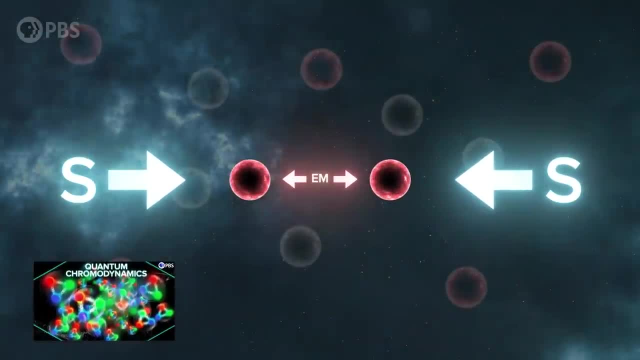 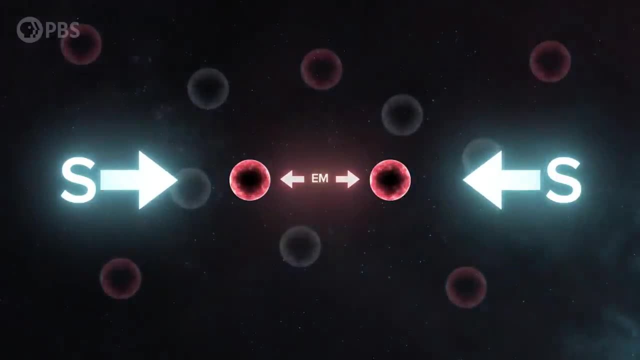 together. We talked about how the strong force holds protons and neutrons together. The story, though, of how it binds entire nuclei is even more complicated. It involves sending virtual quark packets, mesons between the nucleons. So let's take a look. 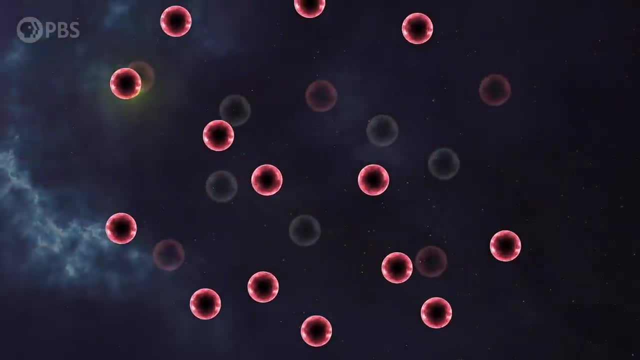 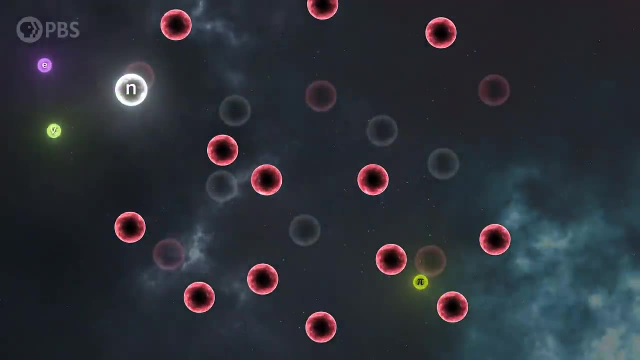 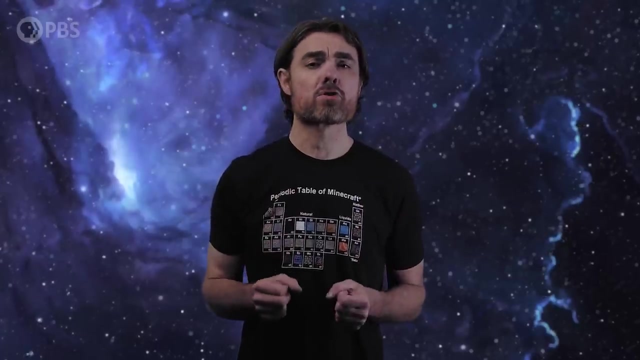 The details deserve their own episode, but the important thing to know is that it's a short-range effect. If a nucleus gets too big, the strong force can't keep things together and various types of nuclear decay become inevitable. Although the strong force vanishes quickly, its strength doesn't change much over the 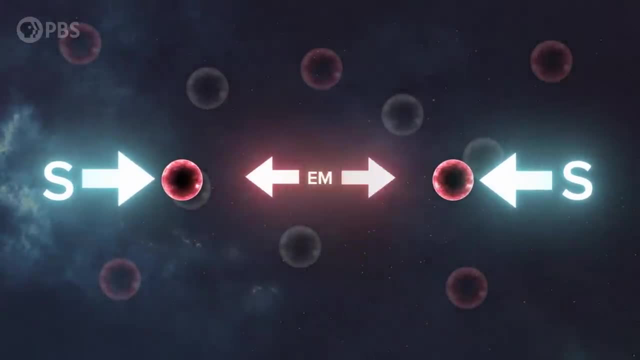 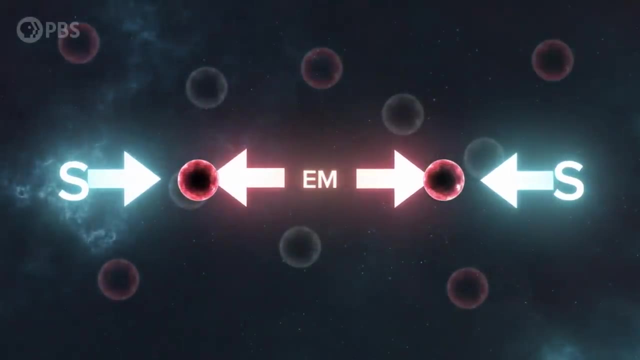 short distance. where it actually works, However, electromagnetism just keeps getting stronger, the closer the two electric charges get. That means electromagnetism can't keep things together. Electromagnetism can overwhelm the strong force if protons are too close together, which 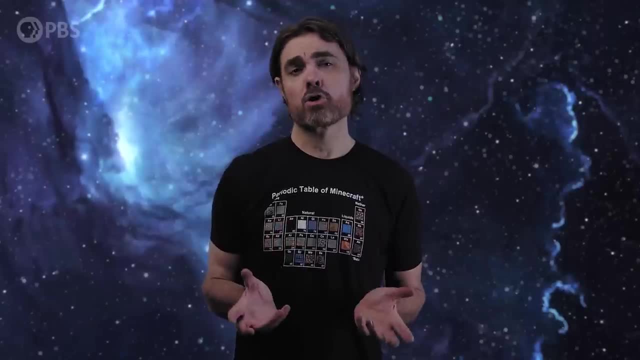 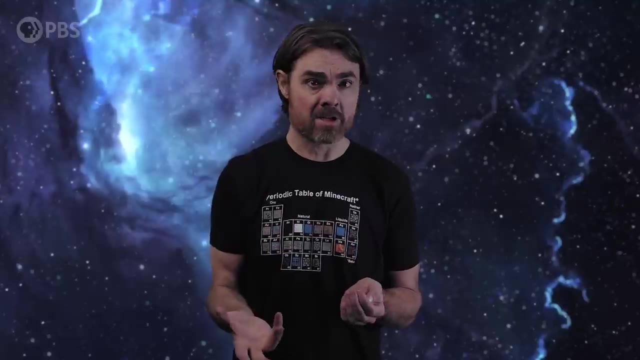 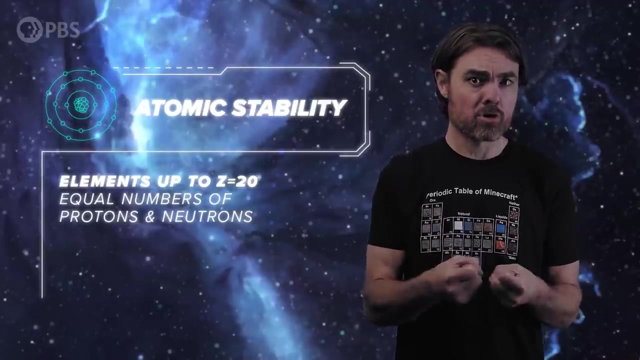 is another way to destabilize the nucleus. That's why neutrons are so useful. They help separate protons so that the strong nuclear force stays stronger than electromagnetism. For smaller nuclei, up to atomic number 20,, an even split of protons and neutrons is usually. 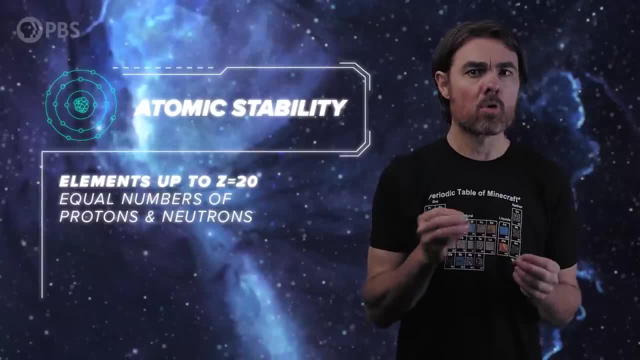 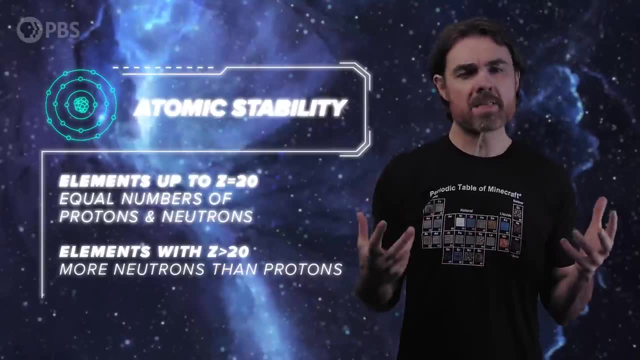 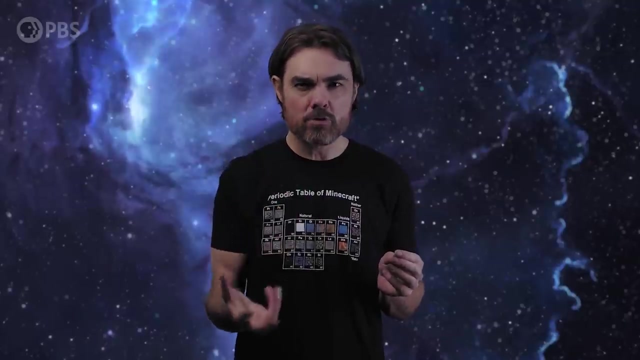 the most stable. But for heavier elements more and more neutrons are needed to provide that buffer, Reaching a neutron to proton ratio of 1.5 or more. But this is only part of the picture. It doesn't explain why the differences of a single neutron can mean a huge difference. 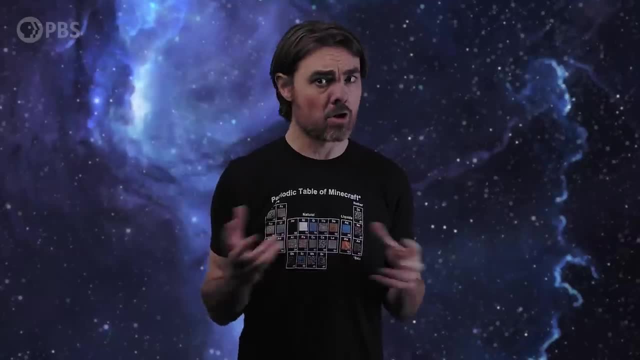 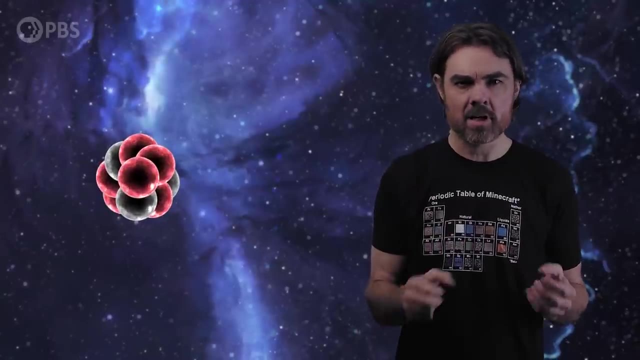 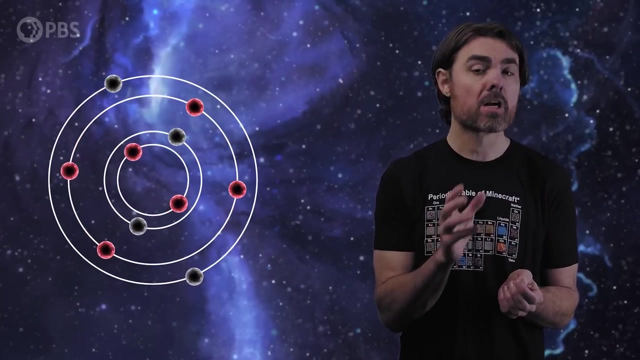 in stability. It also doesn't explain why there's no stable isotope of technetium. To understand that, we have to move beyond the common representation of the nucleus as a muddled blob of protons and neutrons. We have to think of these nucleons as having energy levels. Just like electrons do. You may remember the octet rule from your chemistry classes: If an electron shell has 8 electrons, it's stable. That's the reason the noble gases don't interact with anything, because their electron shells are already complete. 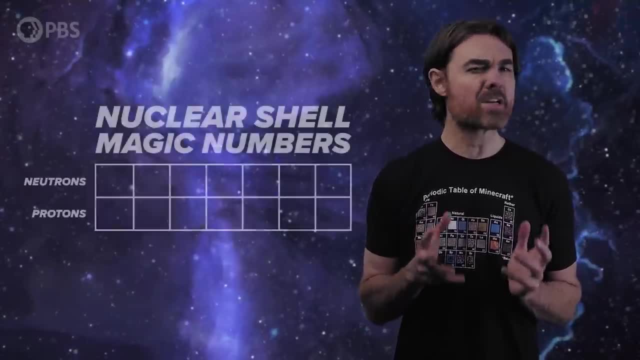 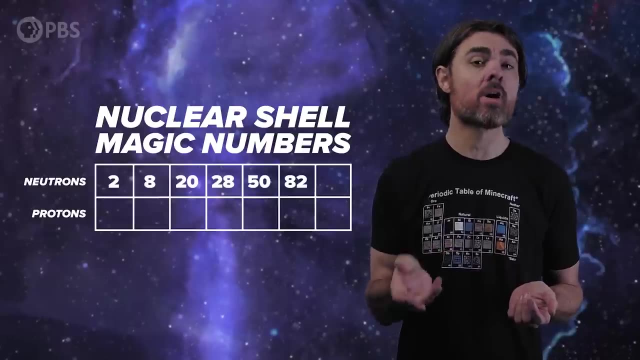 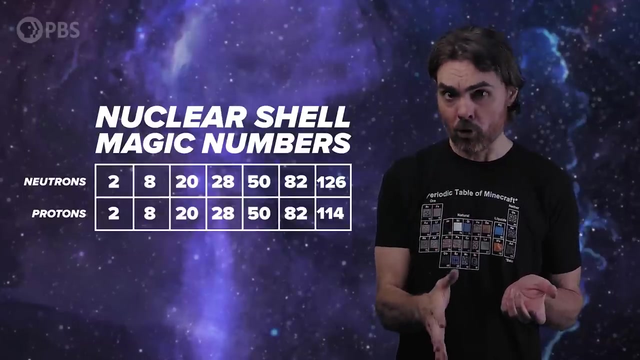 Something similar happens in the case of the nucleus. There are magic numbers which complete nuclear shells. They are 2820, 2850, 82, 126 for neutrons And 2820, 2850, 82, 114 for protons. The closer a nucleus is to those numbers, the more stable it'll be. 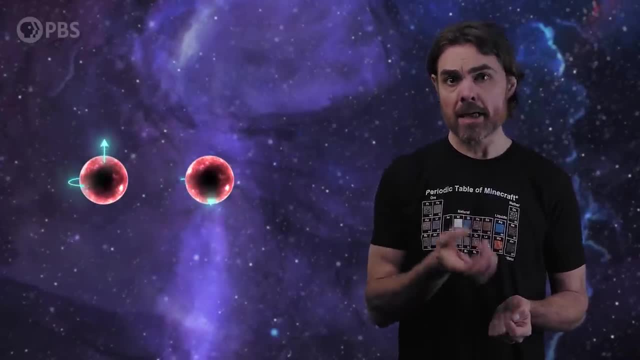 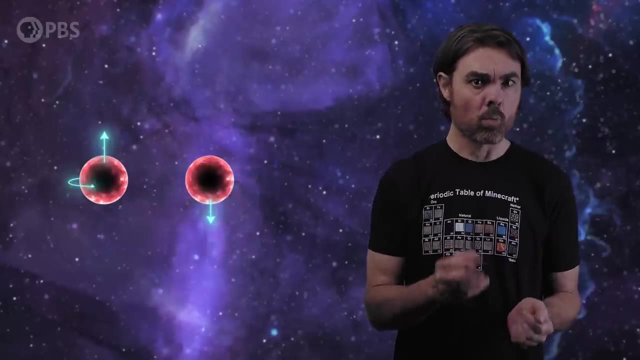 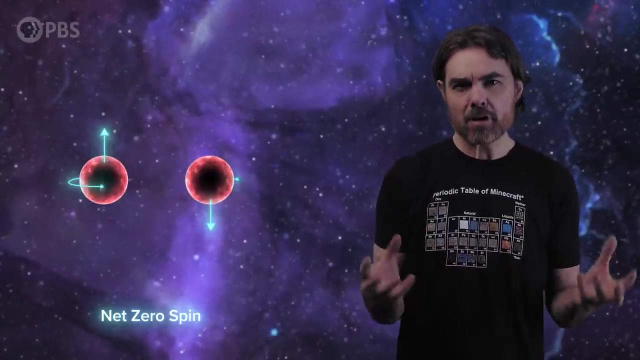 The magic numbers, as you might have noticed, are all even, And that's because these nucleons pair up according to their quantum spin, Just like electrons in their shells. One spin up and one spin down results in a net-zero spin. This sort of spin coupling means that even if there aren't a magic number of neutrons, 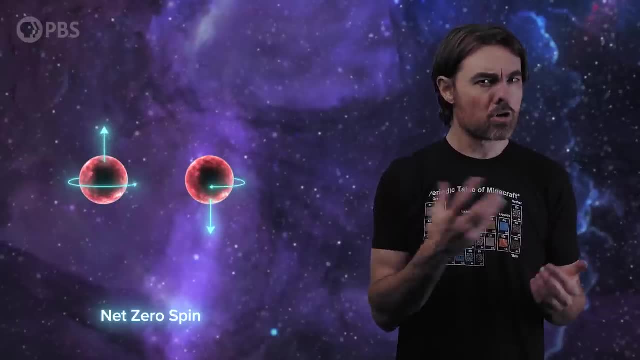 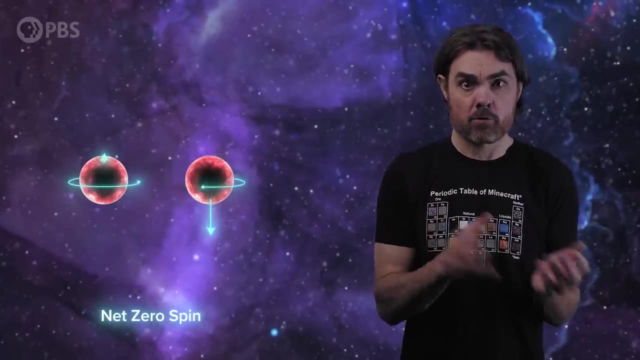 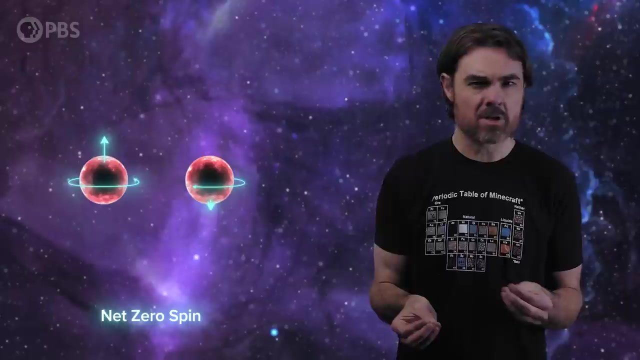 there is a magic coupling. If there is a magic number of protons or neutrons, nuclei still prefer to have an even number of protons or an even number of neutrons, or an even number of protons plus neutrons. Pairs of up-down nucleons form these stable little spin-zero partnerships in so-called 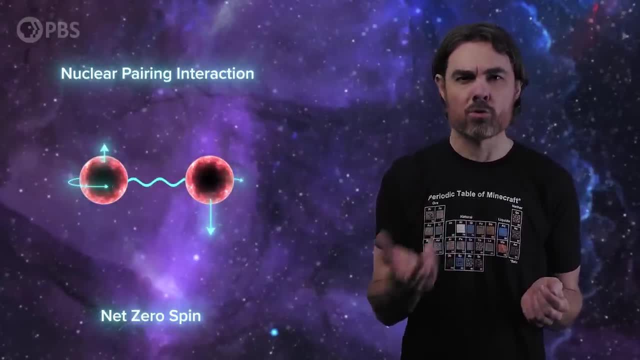 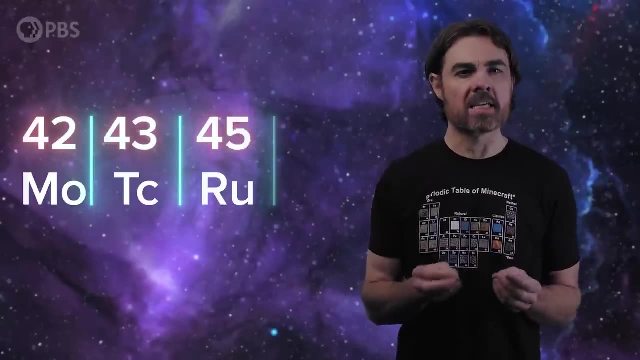 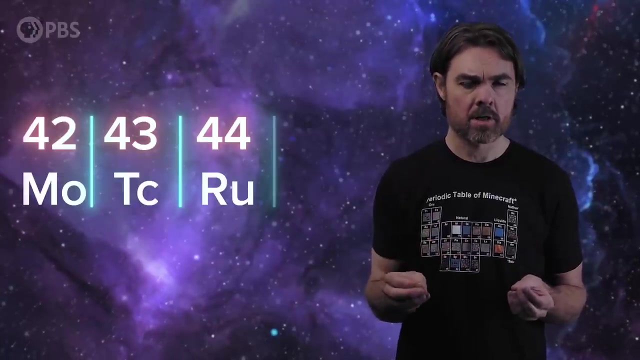 nuclear pairing interactions. Having a rogue proton or neutron with its uncancelled spin seems to be bad for stability. Let's see if we can understand the instability of technetium. Sure, we can see that 43 is not a magic number of protons. 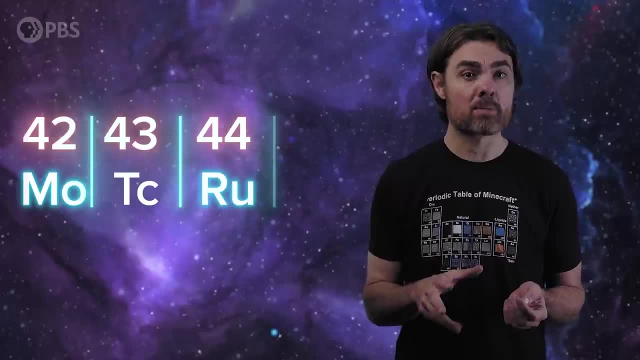 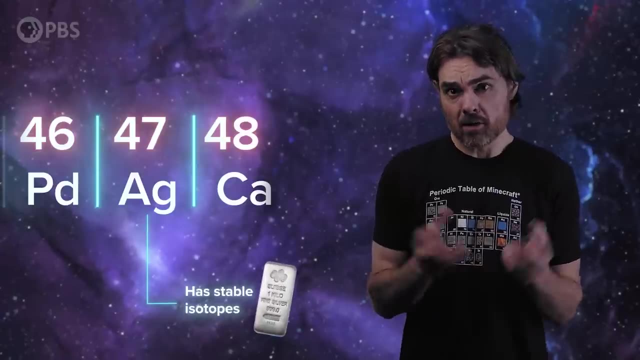 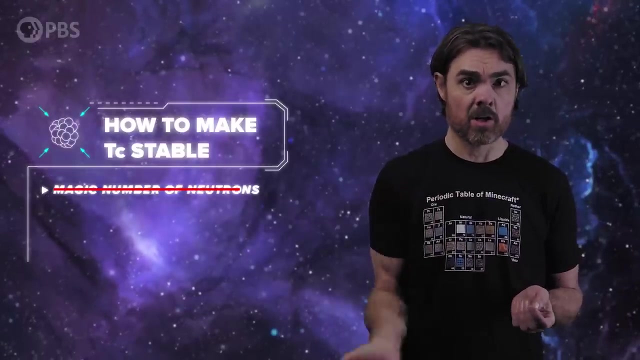 Nor is it an even number of protons like its more stable neighbours molybdenum and ruthenium. But the nearby odd-numbered elements like the 47-proton silver still have perfectly stable isotopes. Even giving technetium a magic number of 50 neutrons doesn't help. Nor does giving it a total even number of nucleons. Why, for example, Technetium-97 survived for 4 million years, but technetium-96 decays in under an hour? It seems there are more mysterious forces at work besides neutron padding nuclear shell. 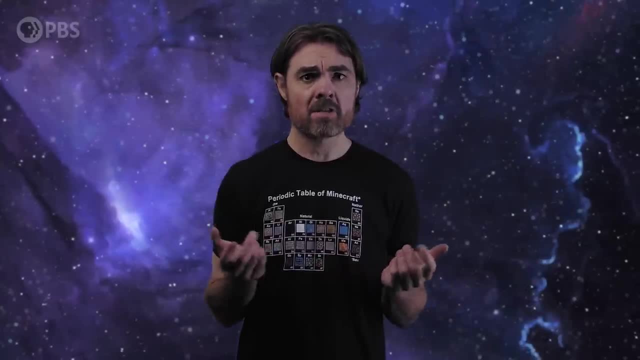 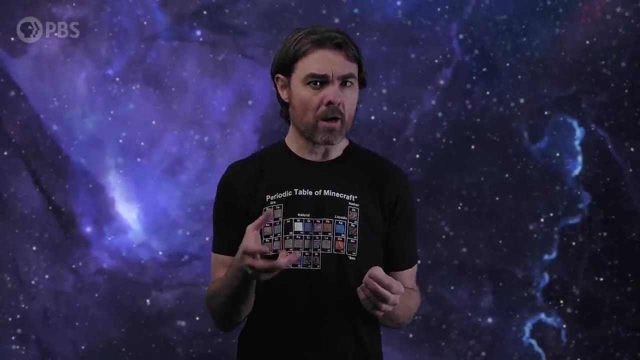 filling and spin coupling. It turns out there is no simple set of principles to determine nuclear stability. There are so many factors at play that the only way to figure this out is to simulate the nucleus, And we've had some remarkable success doing this. 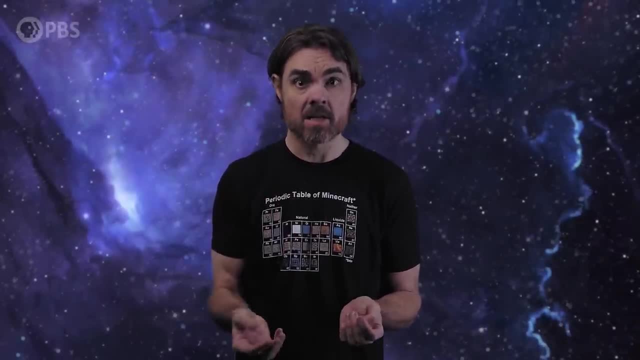 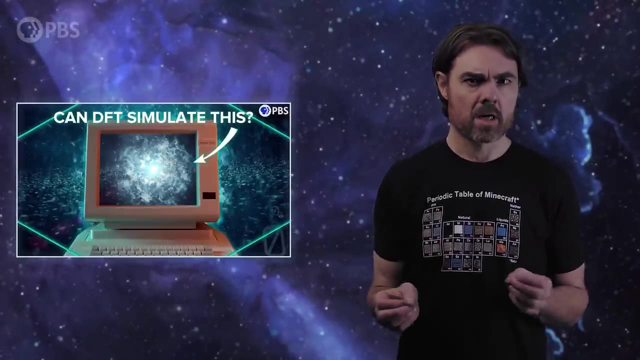 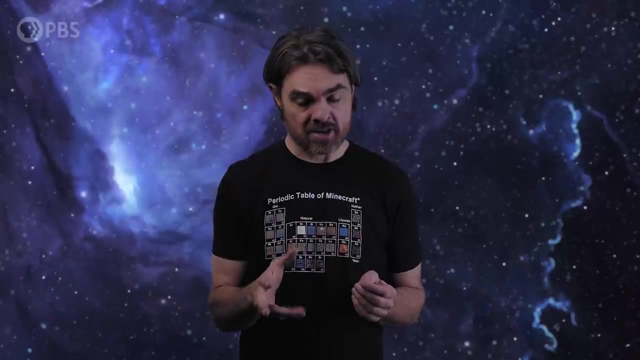 We've had some remarkable success Doing this using computational techniques like density functional theory, which we explained in a previous episode. These models are still not perfect, but they make many predictions that we've verified and some predictions that we haven't verified, For example, the island of stability. 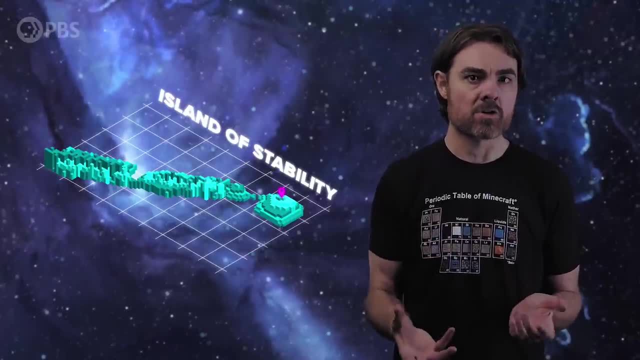 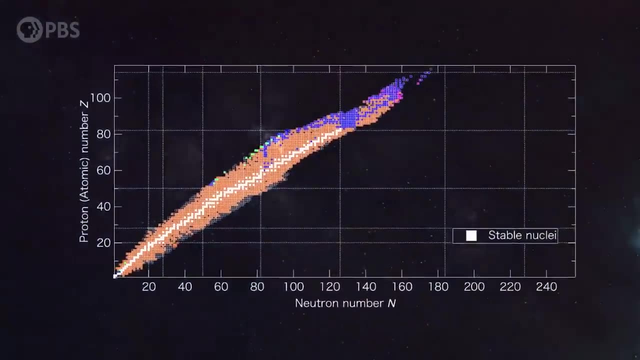 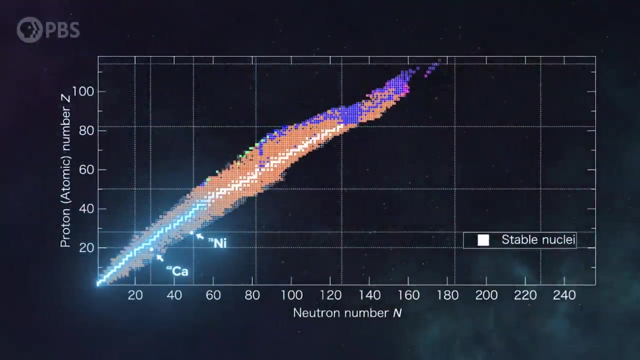 When we combine our experimental data with our simulations, we can make graphs like this one. Here we can see the magic number of protons. The elements with the magic number of protons have more stable isotopes and there tend to be more isotopes with a number of neutrons close to the neutron magic numbers. Patterns emerge, but not so as to give us a clean set of rules for what is needed to yield a stable nucleus. As for the unstable ones, like technetium, they have unlucky spots in terms of not having magic or even even numbers of protons. 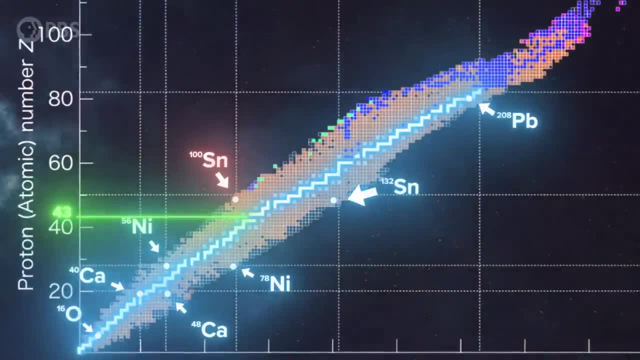 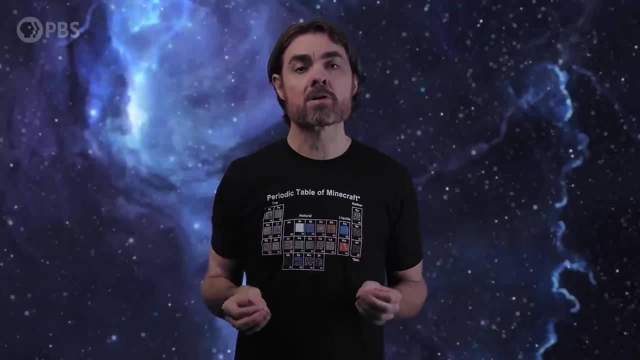 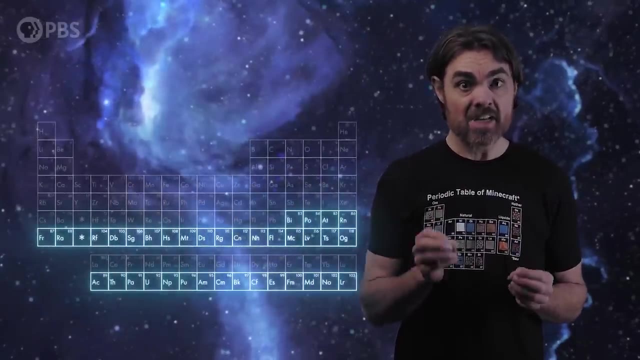 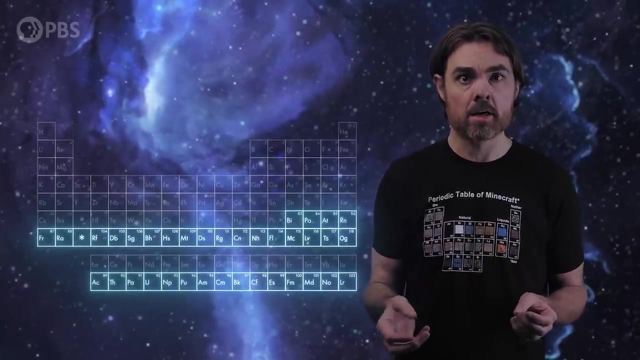 And then, for whatever complex reasons, there is no configurations of neutrons that can stabilize that unhappy nucleus. So are there elements not on the periodic table that humans can or have invented? There are many. Nature can make these, but unless that production process is ongoing on Earth, like with carbon-14,. short-lived unstable elements are extremely rare in nature, only appearing briefly in the decay chain of other longer-lived unstable elements. The first was technetium, but now we've synthesized 24 artificial elements, filling in Mendeleev's gaps and also extending the periodic table all the way to 118 Oganesson. 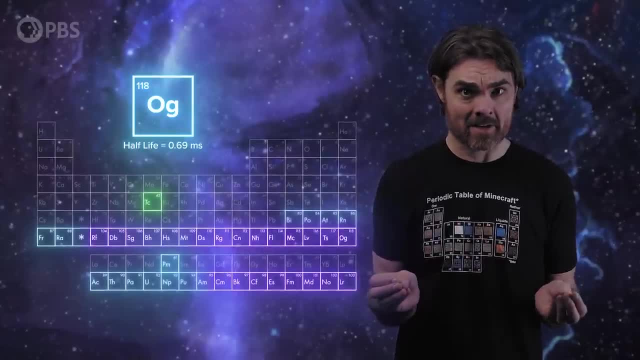 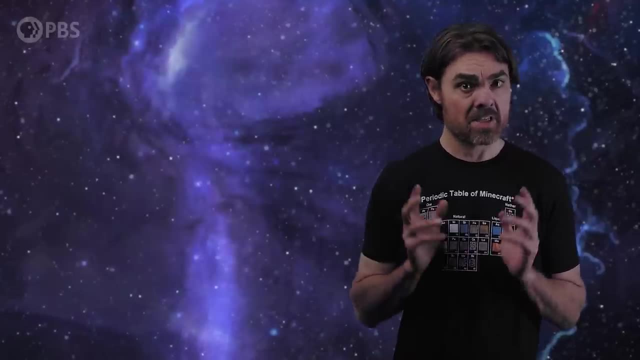 with its half-life of 0.69 milliseconds. There are elements that are not on the periodic table. There are elements beyond that, but we haven't made one last long enough to unambiguously detect them. But this isn't the end. 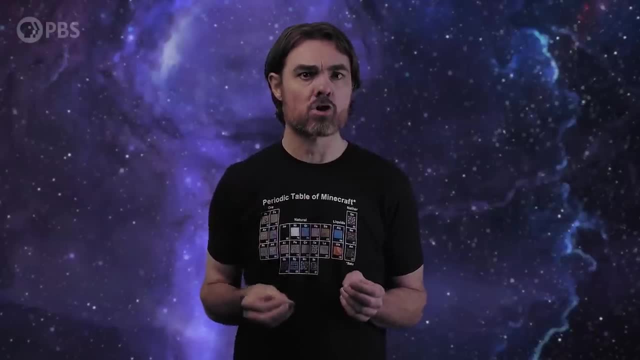 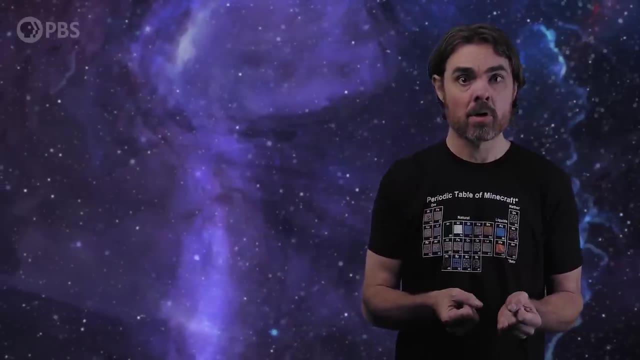 I've hinted at this island of stability. Our calculations show that there may be more magic numbers for large numbers of protons and neutrons beyond the current periodic table, And our computer simulations agree. We aren't sure what these magic numbers are exactly, but apparently they are in the 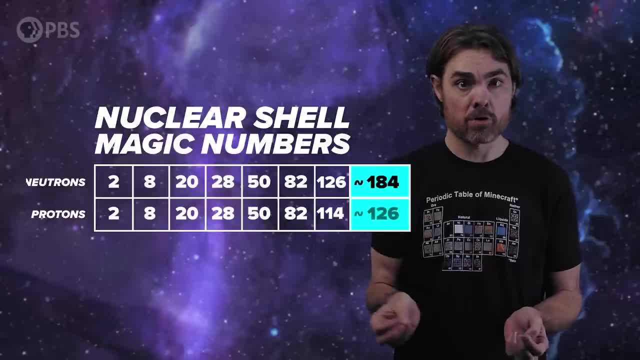 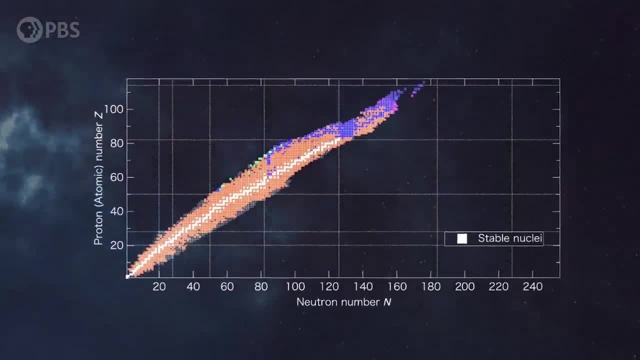 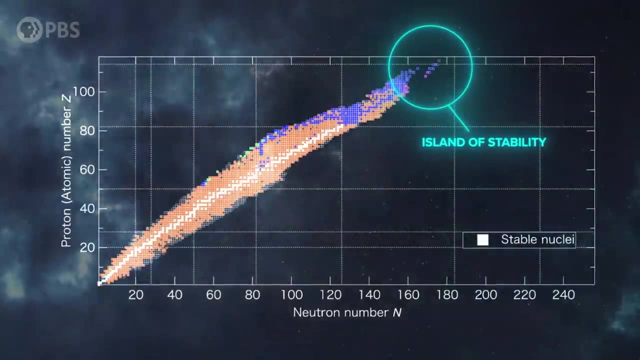 neighborhood of 184 for neutrons and 126 for protons, and they could have half-lives of millions of years. These stable-ish elements would appear here on the graph I showed from before: A small island of stability in an ocean of hopelessly unstable isotopes. 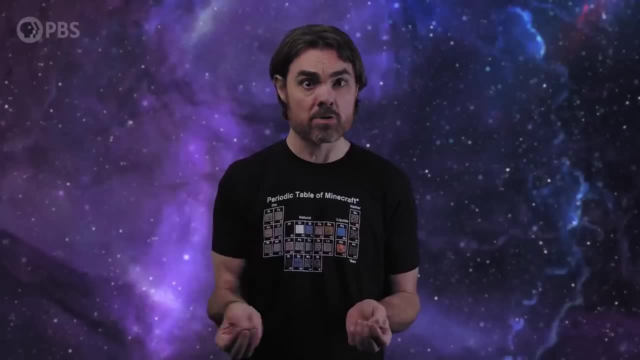 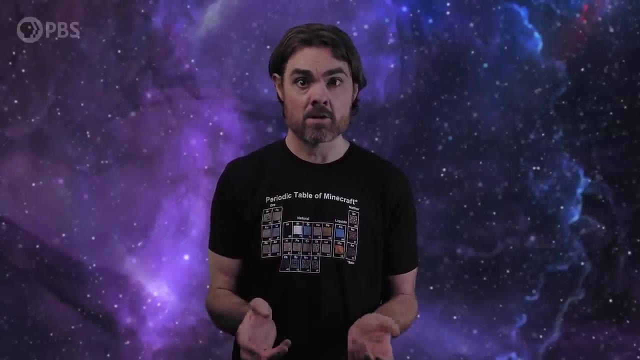 But we've not been able to reach that island with the same techniques we use to craft the other artificial elements. If we want to get there, our conventional nuclear reactors and particle accelerators will not be enough. We will have to come up with something new. 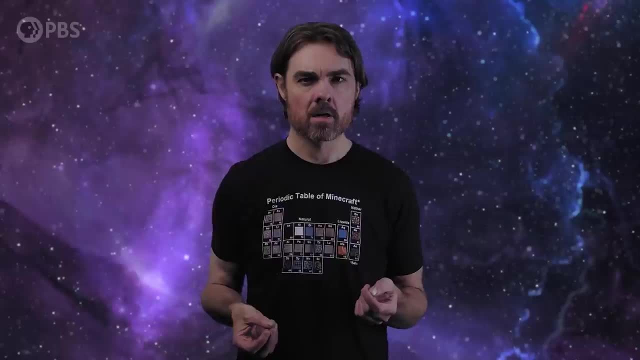 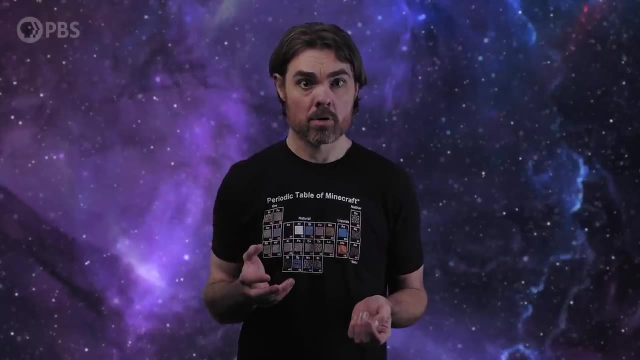 But why should we even try to get to the island of stability? I mean, it's nice to get to name a new element, but other than that, would such a discovery have any impact on the world? Well, probably, and possibly a large one. 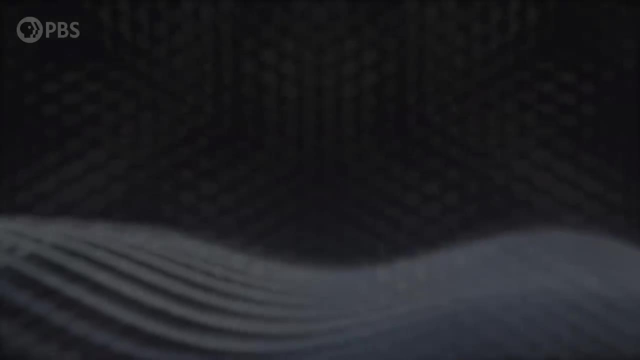 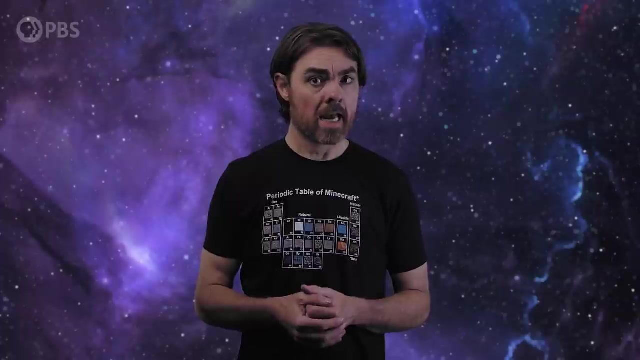 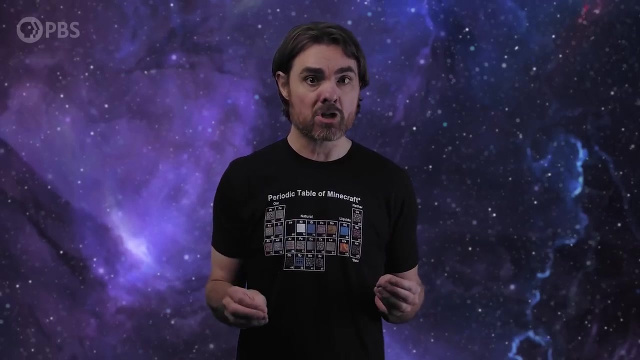 The eras of humanity are named after the materials we had mastered at the time: Stone age, bronze age, iron age, into the current silicon age, And new artificial elements have proved invaluable. For instance, Plutonium is used all the time in medical imaging as a contrast agent. 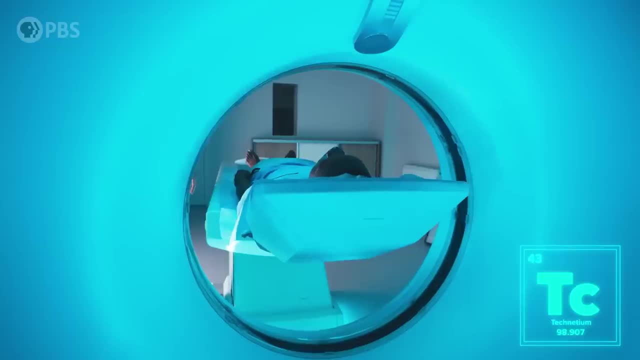 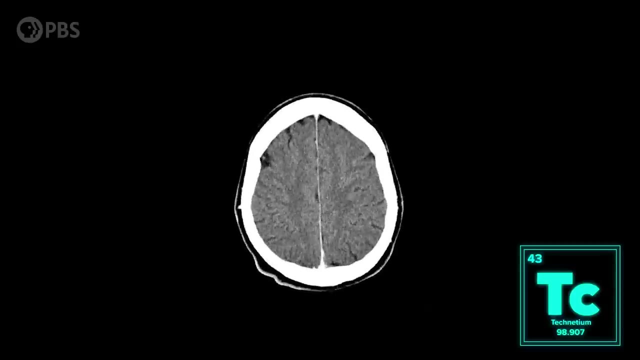 And in this case, its short half-life is actually an asset. By using an isotope with a half-life of only 6 hours, we can greatly reduce the amount of radiation that the patient is exposed to, while also being able to get useful images. 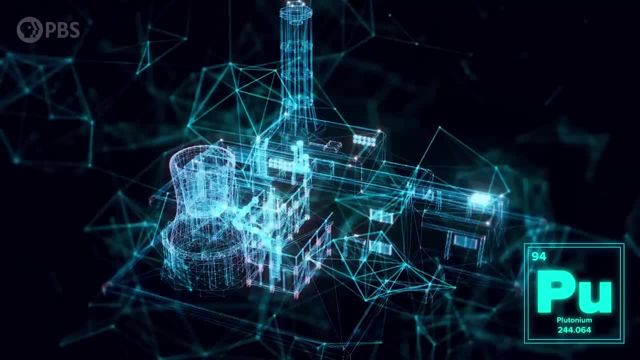 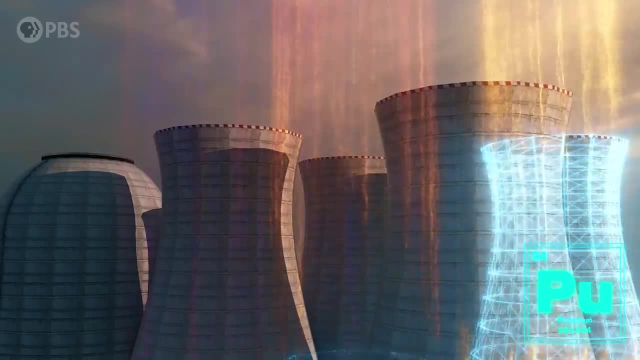 Plutonium is another example. No stable isotopes, but we can breed it from uranium in nuclear reactors, where it becomes a critical part of the fission process in certain reactor types. Plutonium is an example. Hundreds of people rely on it for their electricity. 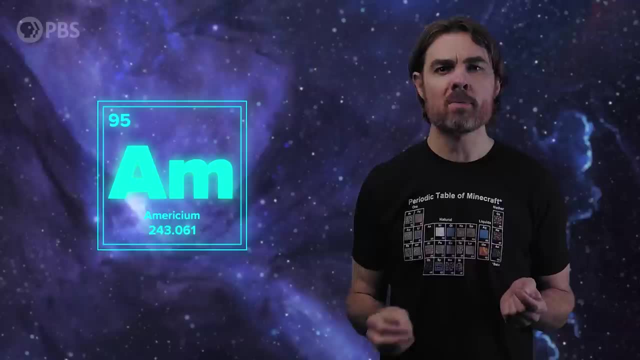 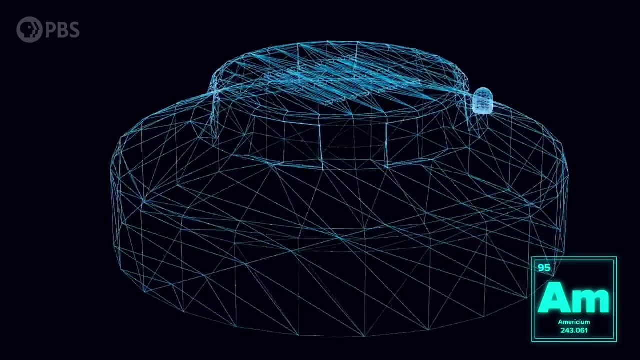 And then there's americium, created by bombarding that plutonium in a cyclotron to kick it one up on the periodic table before a complex chemical extraction process. Americium is critical for smoke detectors, so it's an artificial element that has saved. 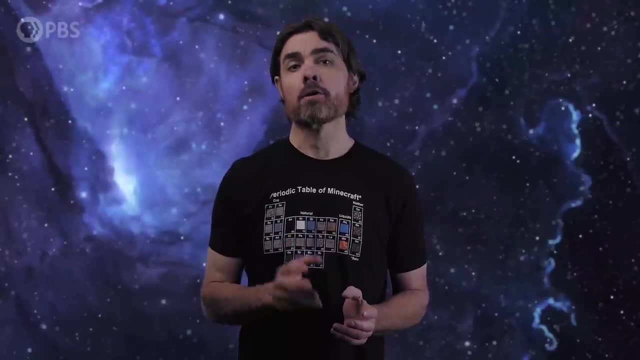 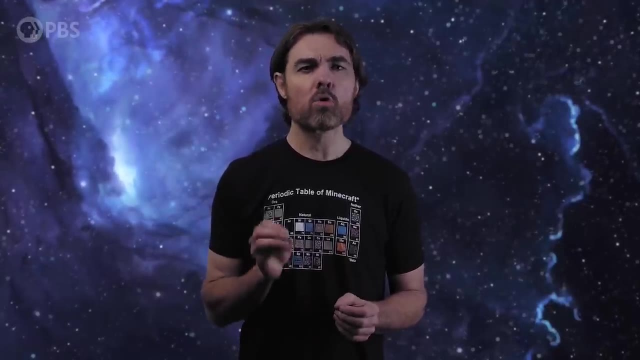 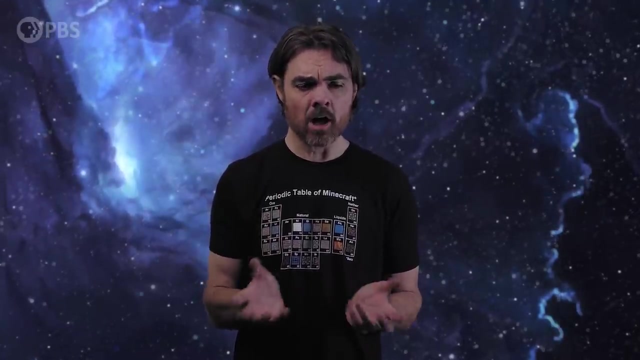 many lives. The elements that we will discover in the island of stability will be very heavy, initially hard to synthesize and somewhat radioactive, But somewhat. People surely have unexpected and perhaps powerful applications. We discover hints of these islands of possibility just beyond the bounds of the known. 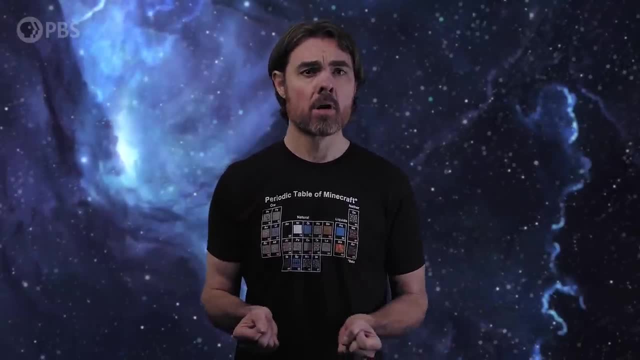 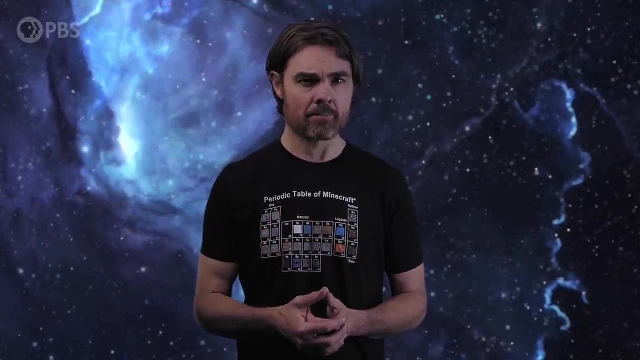 What can we do but hold our breaths and leap towards them, hoping to gain new ground in humanity's journey to further and future horizons of spacetime? As always, a huge thanks to everyone who supports us on Patreon. We seriously would not be here without you. 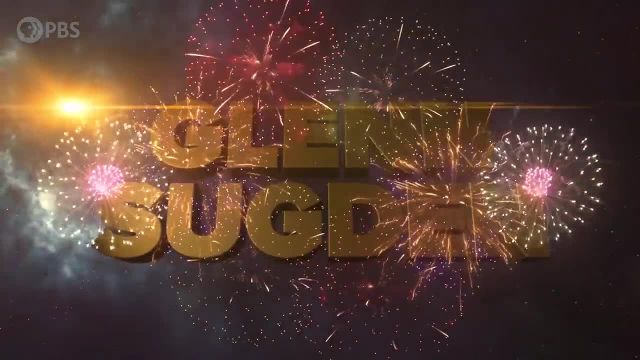 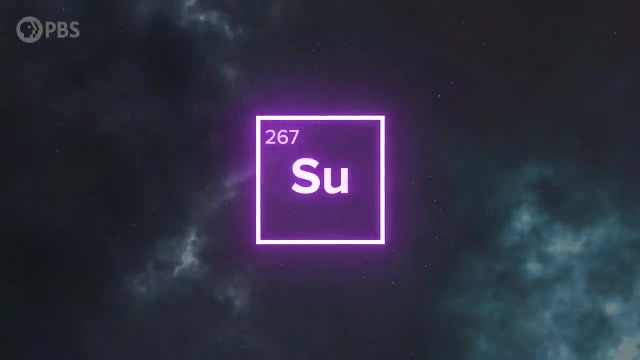 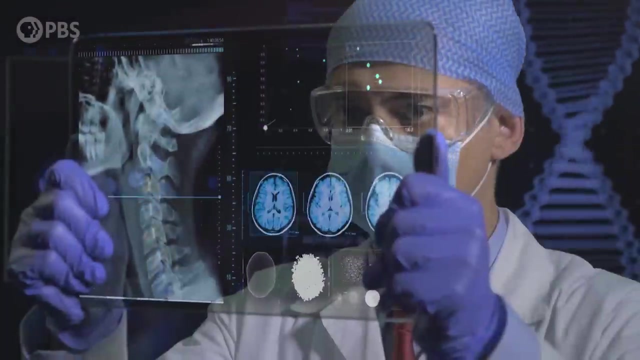 Now A special shout out goes to Glenn Sugden, who's supporting us at the quasar level. Glenn, as thanks for your generous support, we're naming element 267 after you. Sugdenium is great. It's mildly radioactive, extremely useful in medical imaging and is the critical catalyst. 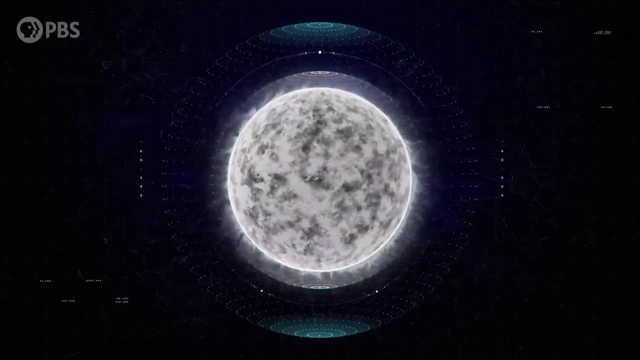 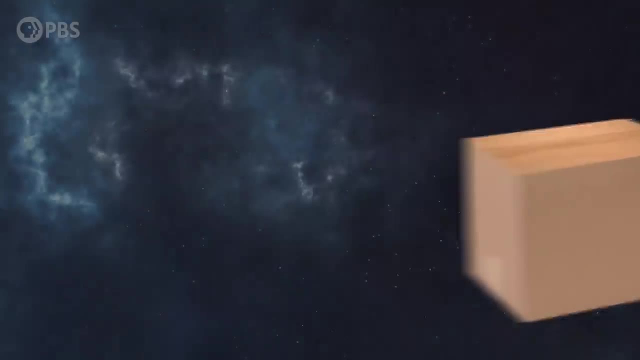 for low temperature fusion. On top of all that, it glows a lovely shade of violet. Glenn, thanks for your support. We'll ship you a gram of Sugdenium as soon as it's invented. Subtitles by the Amaraorg community. 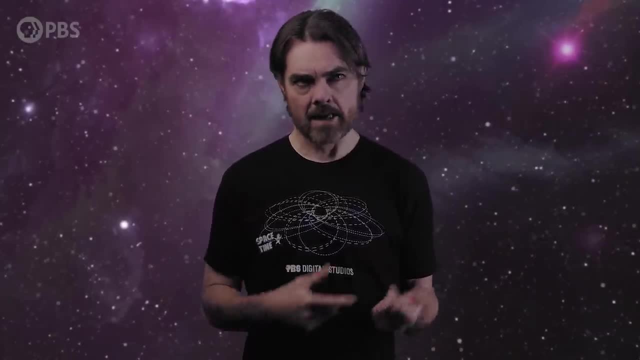 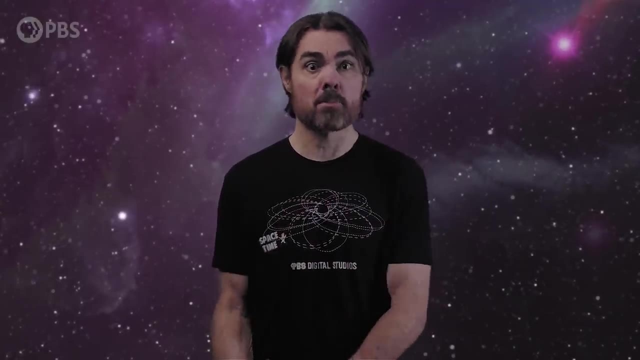 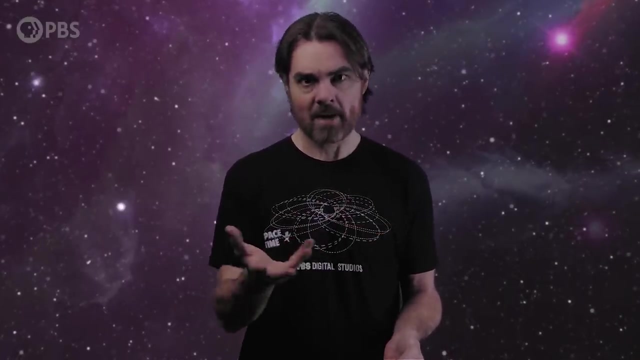 In our last episode we talked about grabby aliens. That's the hypothesis that says that the future emergence of new civilizations has to be cut off at some point, or else humanity is too surprisingly early in the universe, And the cut off is when the universe gets fully colonized by- yeah, grabby aliens. 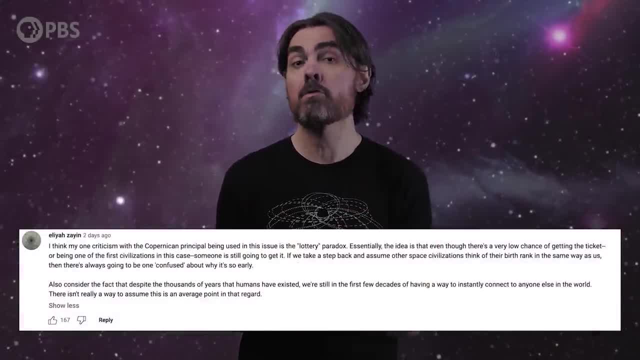 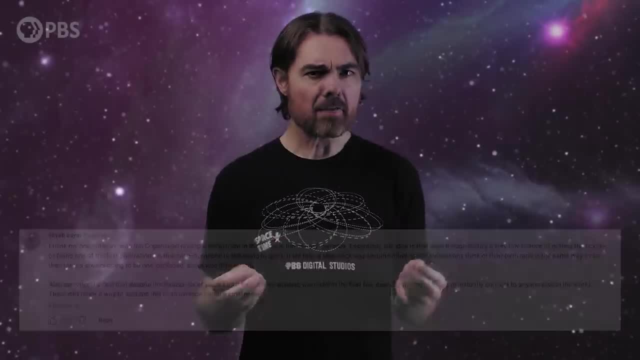 Alaea Zayn has a thoughtful criticism of the use of the Copernican Principle to argue that we can't be especially early in the universe, To paraphrase: Even if there's very low chance of any given civilization being one of the first, someone has to be. 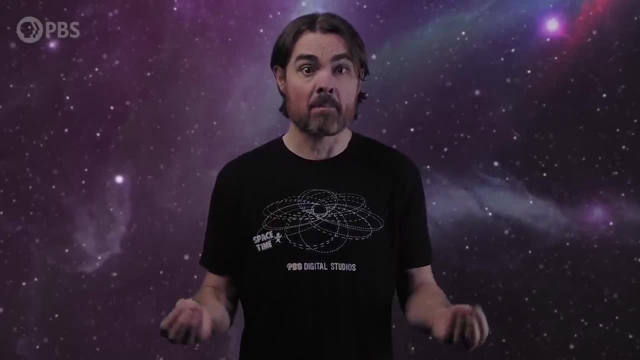 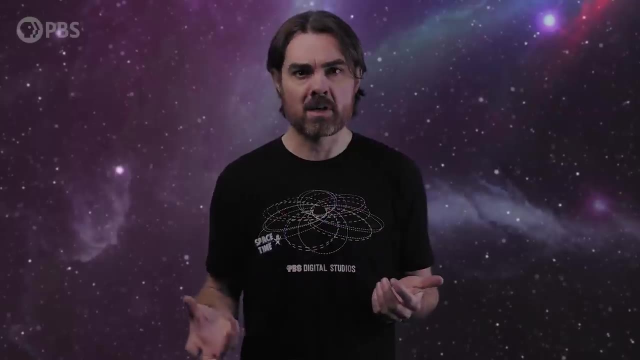 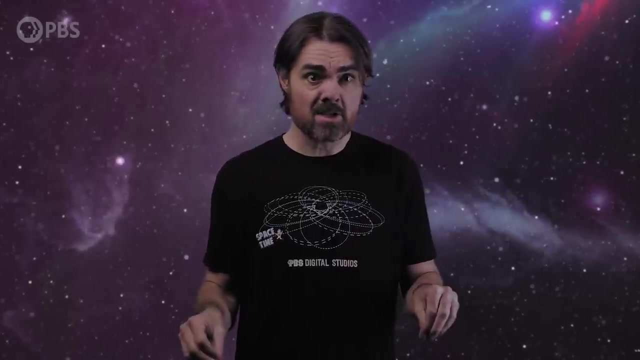 first. so there's always going to be one civilization that ends up being confused about why it's so early. So here you get to one of the most contentious aspects of anthropic reasoning If I argue that I should find myself in the most typical circumstances consistent with my existence. 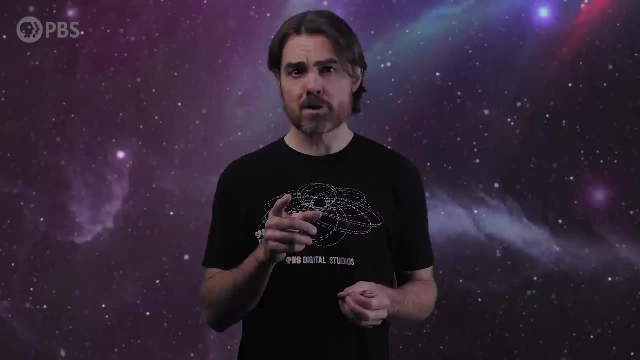 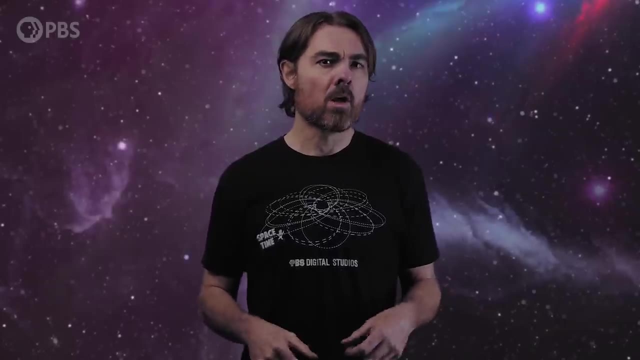 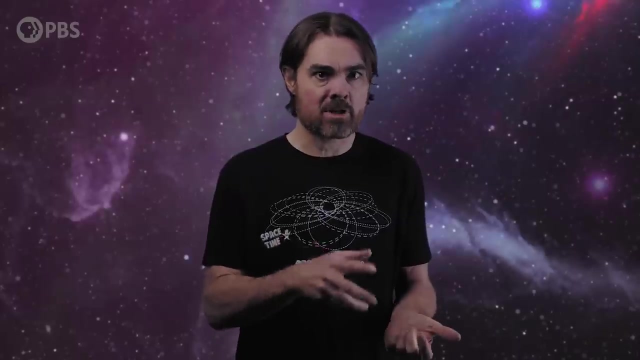 what circumstances does that preclude? Nick Bostrom's self-sampling assumption tries to clear this up. It says that, all other things being equal, an observer should reason as if they are randomly selected from the set of all actually existent. so past present. 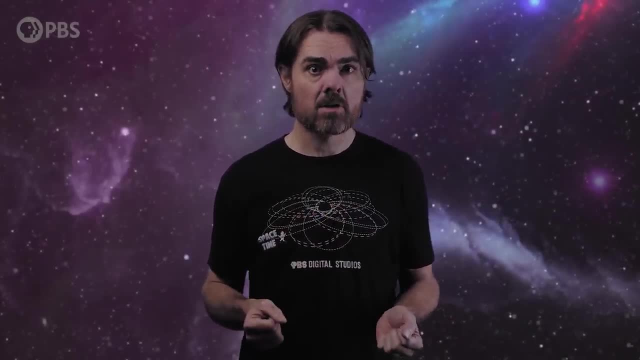 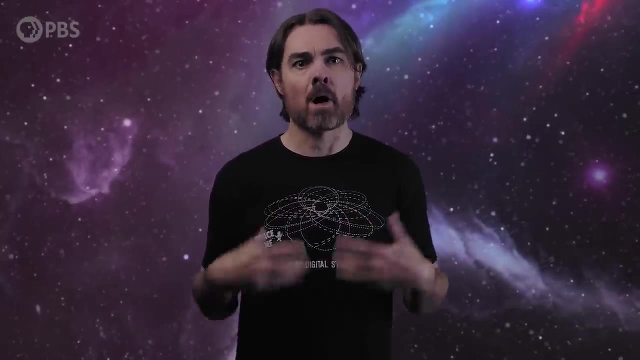 and future observers in their reference class. So the trick, then, is figuring out what your reference class is. For example, if I define my reference class as a biological being, then I don't have to be surprised that I don't find myself somewhere uninhabitable. 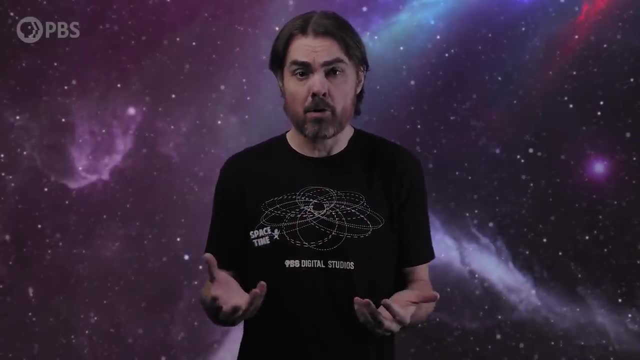 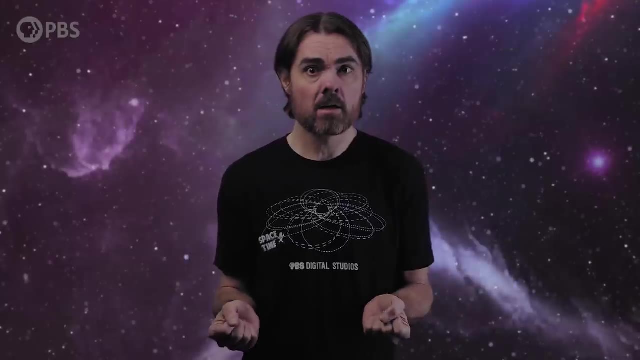 But that permits the forbidding. I'm lucky to have a 4 billion years of habitability on the Earth prior to my birth. So then, why am I, in the least brutal of those 4 billion years? Just lucky? But if I define my reference class as those who are able to formulate anthropic arguments, 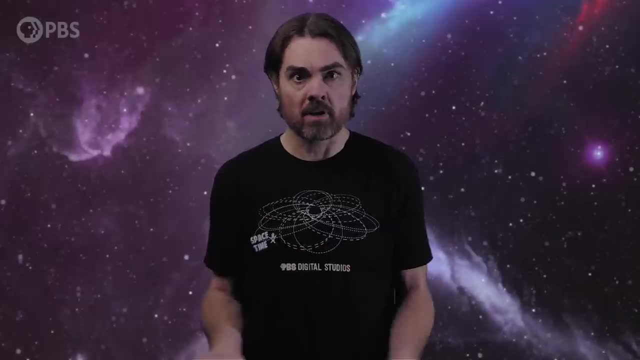 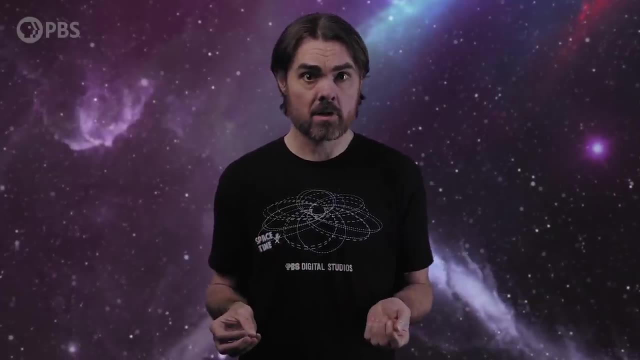 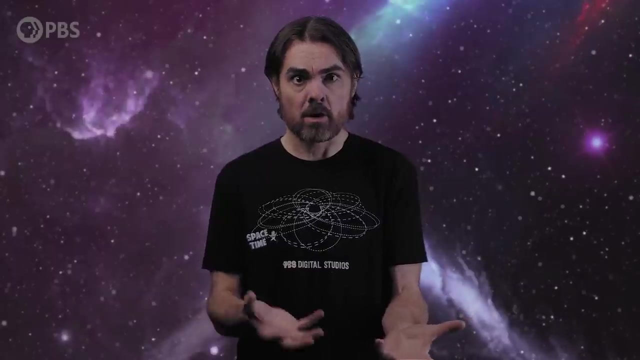 then it's less surprising that I live in a modern civilization. But then why can't I define my reference class as those who observe an empty universe? After all, I am. my mental experience, The fundamental experience of seeing an empty universe, is what got me asking these questions. 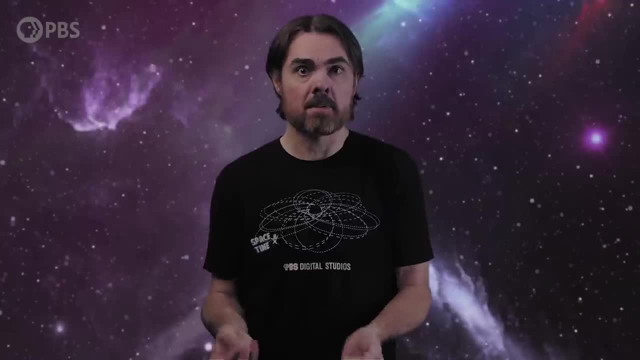 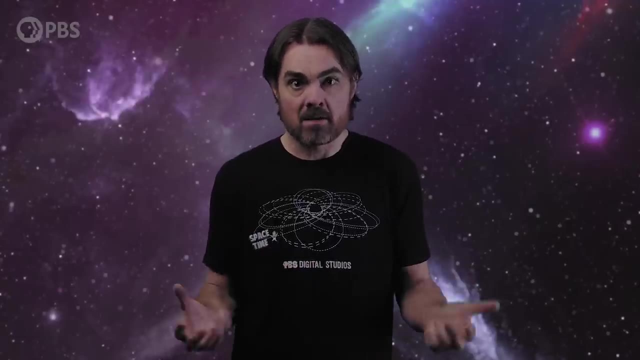 in the first place. Being a member of an early species is one of the few circumstances consistent with what I am. You could say this is too restrictive a way to define your reference class, but the fact is there is no clearly correct way to do it. All of this anthropic.